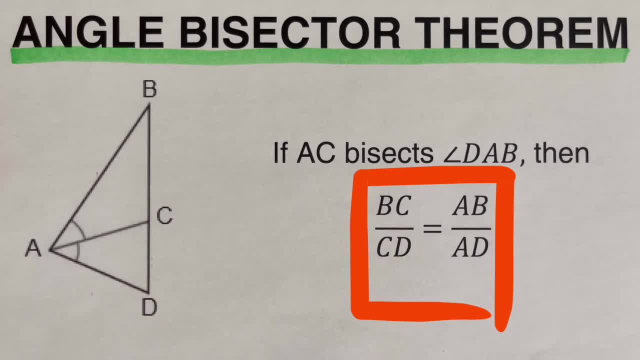 angle bisector theorem. Now please take note that these letters A, B, C and D are variables. It has to be A, B, C and D in all problems And at the same time we also remember that, even if we 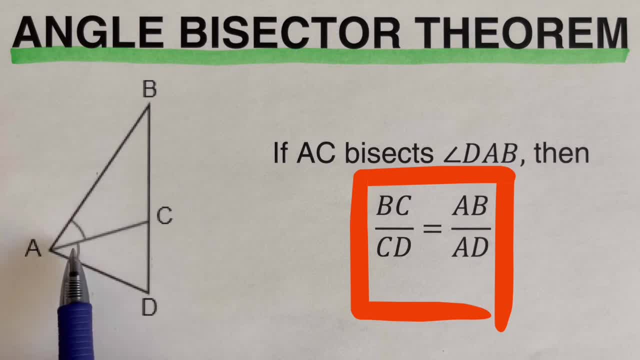 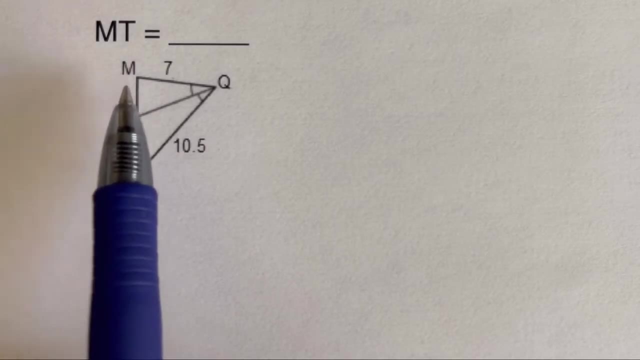 rotate this picture as long as we get an angle bisector, then we can go ahead and use this angle bisector theorem that we have right here. Now let's take some examples. Looking at this first example, right here, we're supposed to determine the measure of MT. Now please remember that this: 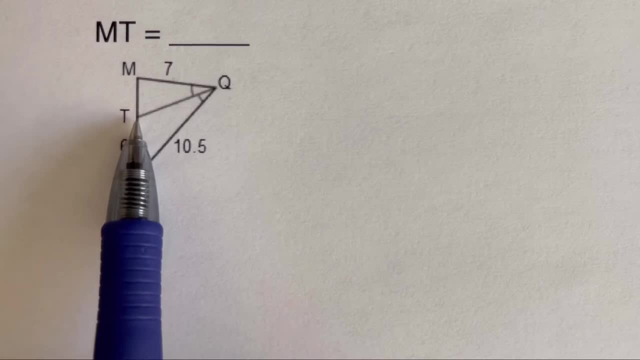 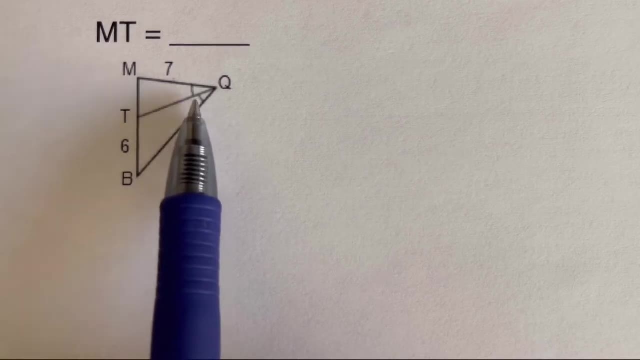 TQ or QT line segment is an angle bisector. We can see that by the label right here on the corner. these two angles are equal. So then we can go ahead and say that this is an angle bisector. It divides angle Q into two equal parts. From here we can go ahead and say that MT, that's the. 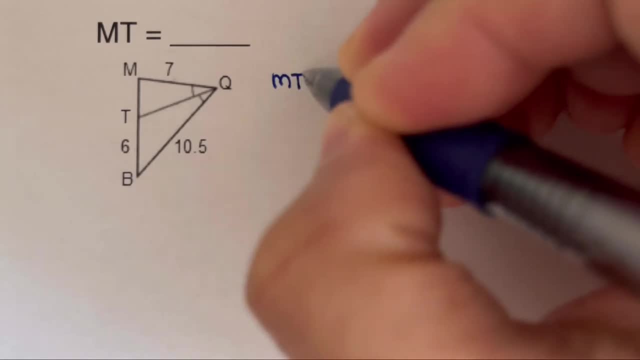 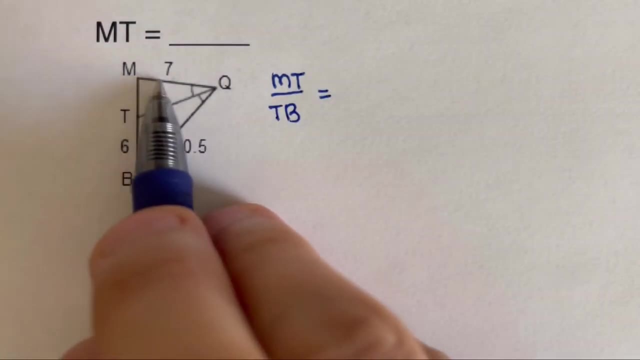 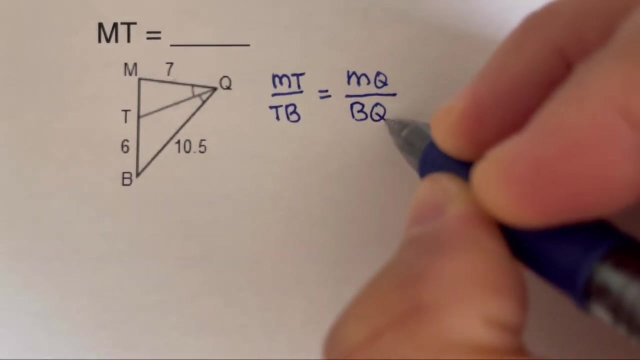 first one right here, So I'm just going to write that down here. So MT over the other half, which is TB, is equal to QT. So this is the angle bisector theorem. Now let's take a look at this example. So TQ is equal to, that's MQ over the one on the other side is BQ. So that we can go ahead. 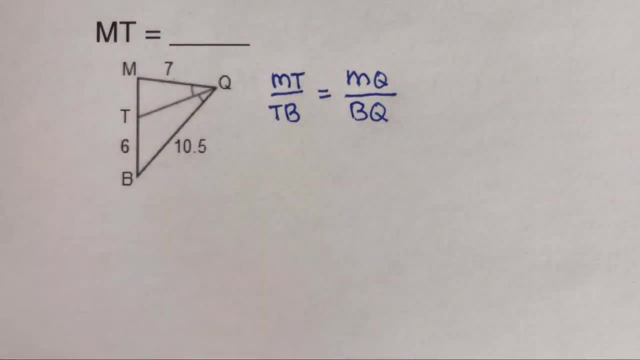 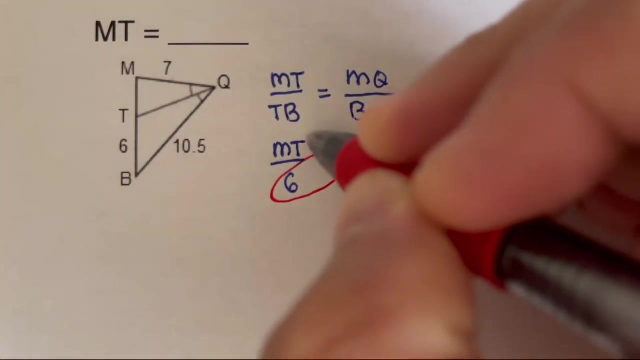 and plug the values in. So our MT is missing. So we can go ahead and just write MT over there over. our TB is six and that is equal to our MQ is seven over our BQ is 10.5.. And then again we are supposed to solve for segment MT here so that we can go ahead and cross multiply these two and cross multiply these two so that we can go ahead and rewrite this as 10.5.. 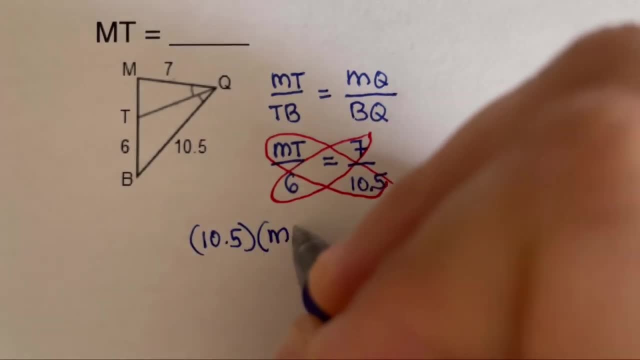 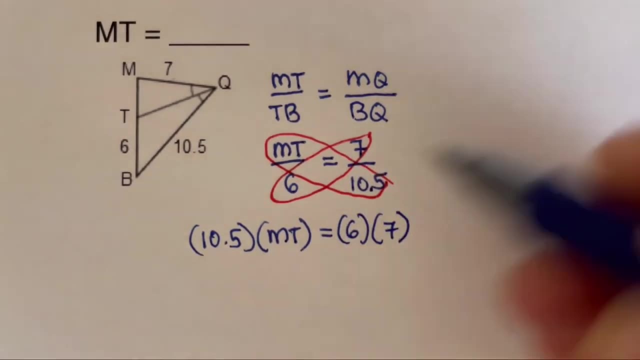 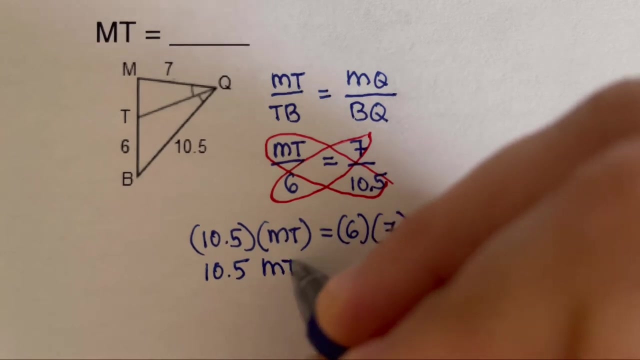 That's going to be paired up with MT is equal to that. We multiply these two together, So that would be six times seven. So six times seven is 42.. So that is 10.5.. And then that's: MT is equal to 42, because six times seven is 42.. 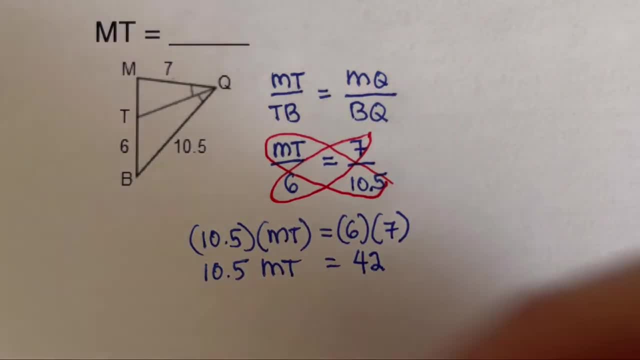 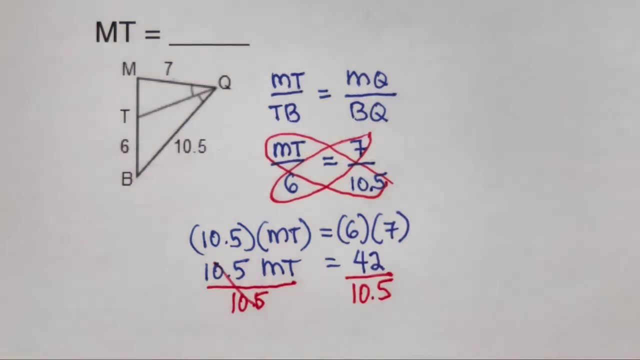 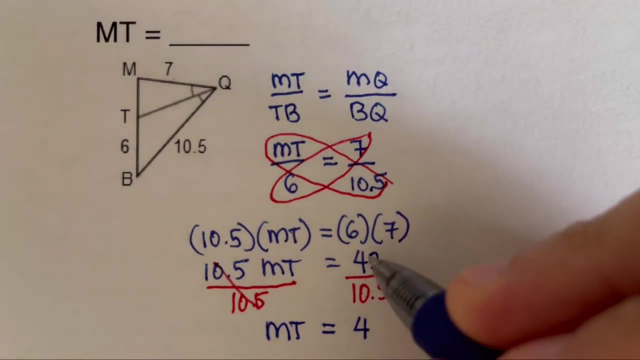 So that if we want to solve for segment MT, we can go ahead and divide both sides by 10.5 and divide this by 10.5.. So we are left with MT. So then our value for MT here is four. So if you divide for 42 divided by 10.5.. 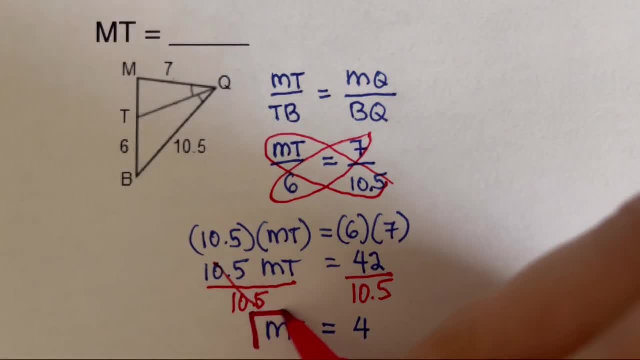 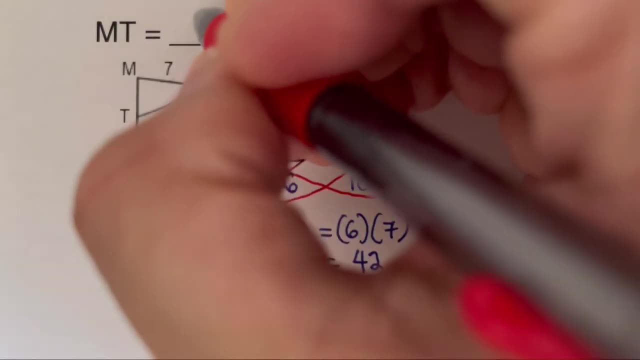 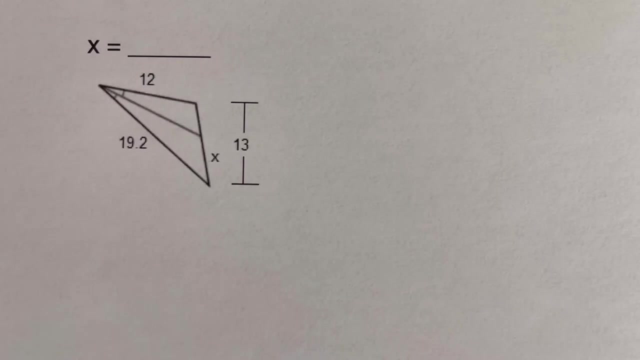 The value is four. So this line segment that we have up here is four. So we can go ahead and write this value for MT here as four. Now let's move on to the next example. At this time, I would encourage you to pause this video and try this problem out on your own. 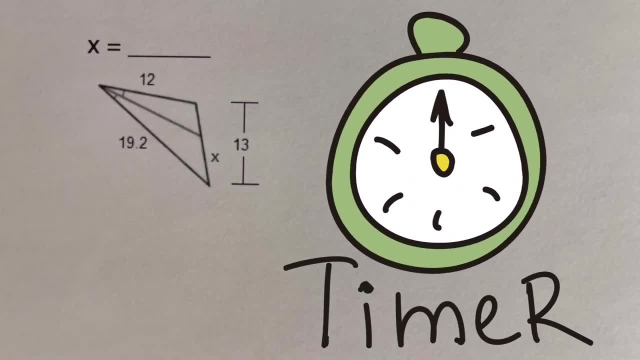 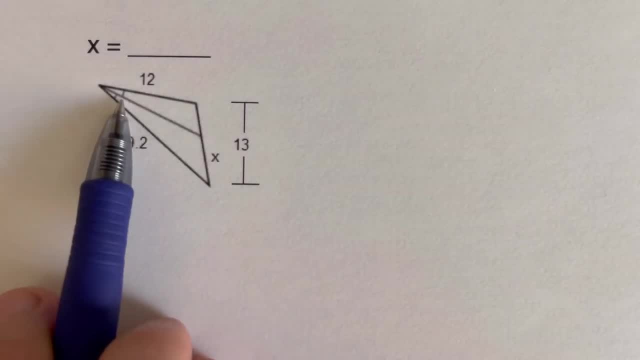 And when you're done and pause it and check your answer. Okay, so we go over the problem here. So again, this line segment that we have right here is an angle by sector. We can say that this is an angle by sector because it divides this corner right here or this angle into two equal angles. 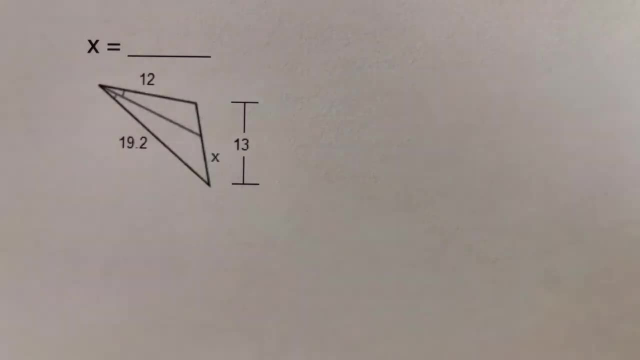 So then we go ahead and say that this is the angle by sector. We can go ahead and set up the equation here. So that means this first piece divided by the second piece is equal to this piece right here divided by this piece right here. 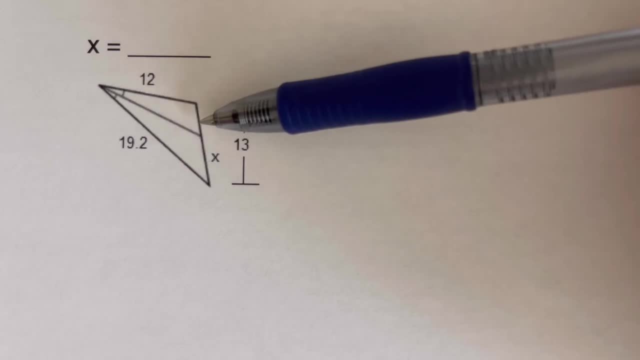 But the thing is, this piece is not equal to this piece right here. This piece is missing. However, we know that from this end to the other end is 13. We can therefore say that, to get the measure for this, that would actually be the whole thing. 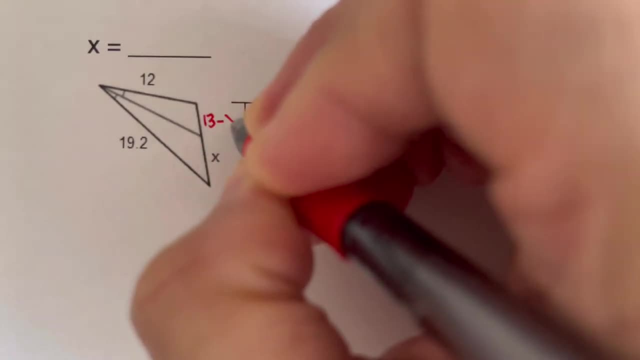 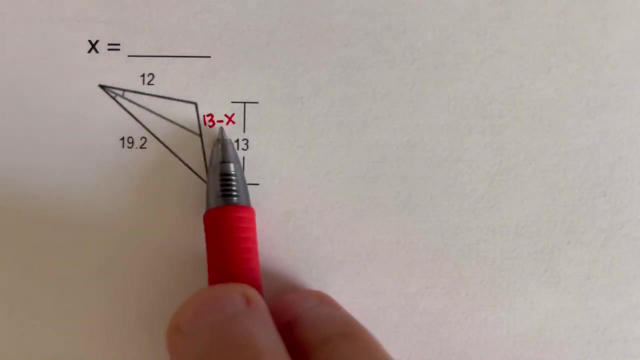 which is 13 minus X. So, whatever the value of X is if we subtract it from 13,. that is this measure right here, so that we already have a label for both of these segments here, so that we can go ahead and set up the equation. 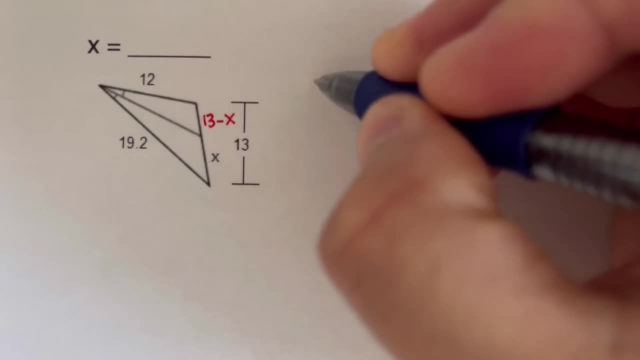 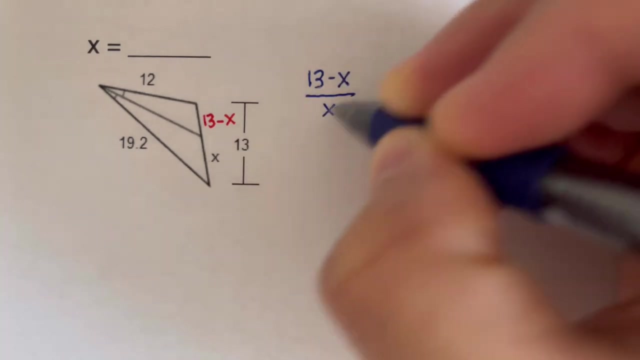 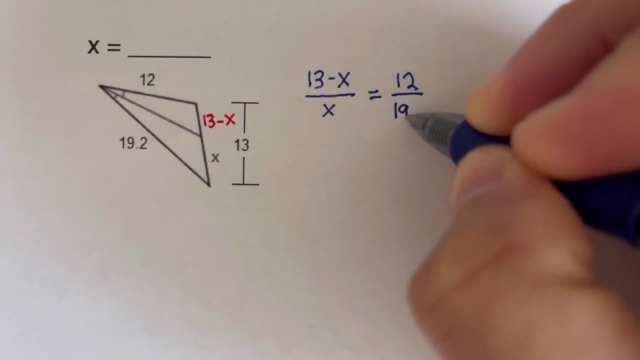 Again the first piece divided by the second piece, So that is 13 minus X over the second piece is X equals- We have the first piece on top right here- is 12 over 19.2.. So that we go ahead and cross, multiply these two together. 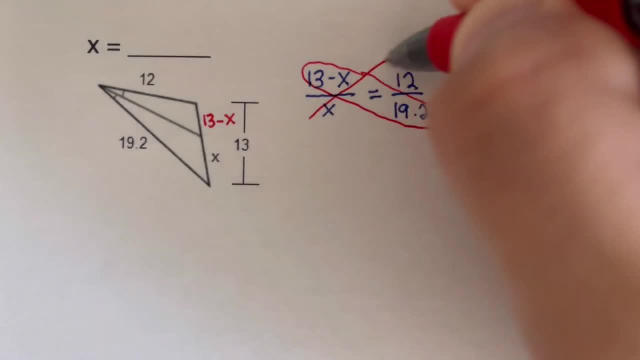 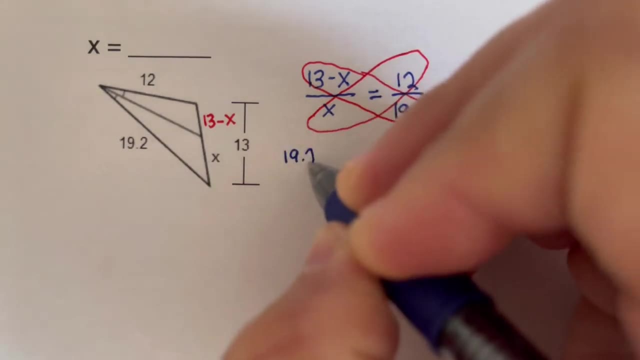 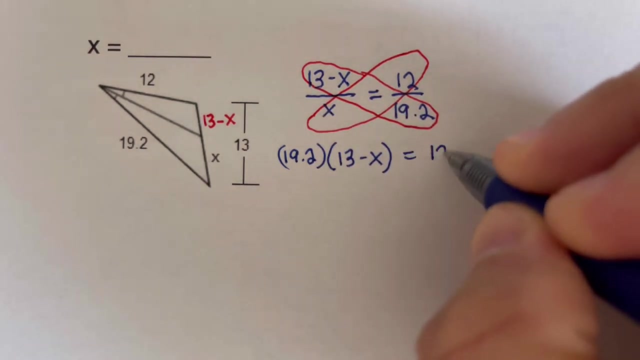 So these two are going to get partnered up, These two will partner up as well, so that we are able to come up with that's going to be 19.2.. 19.2 times 13 minus x. i paired them up and that is equal to 12 times x. 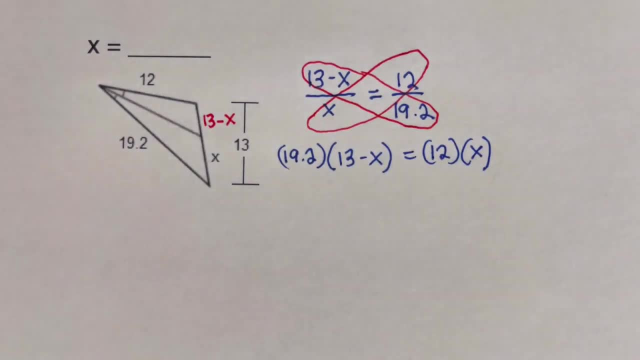 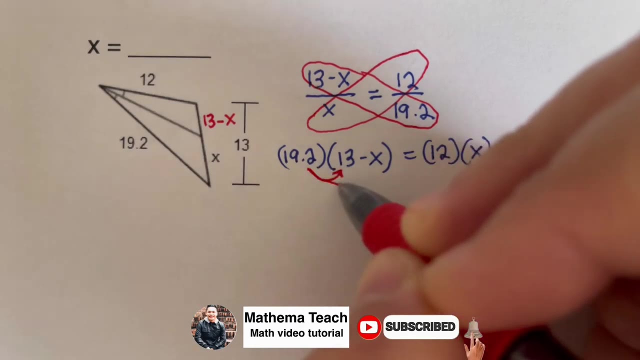 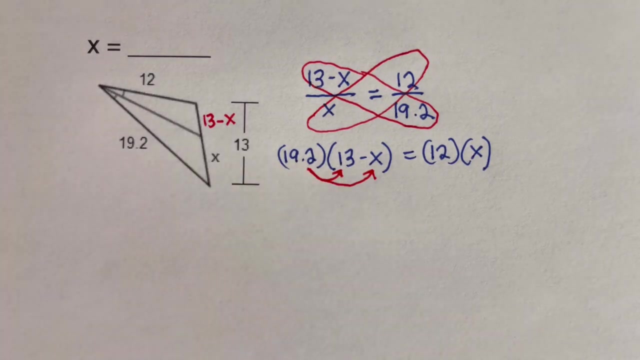 so that we go ahead and distribute this um 19.2 to each of the terms inside the parentheses. so distribute, multiply it with that. multiply it to the x as well, so that we go ahead and say: 19.2 times 13 is 249.6. so that's 249.6 minus 19.2 times x is 19.2 x, and that is equal to 12 x. 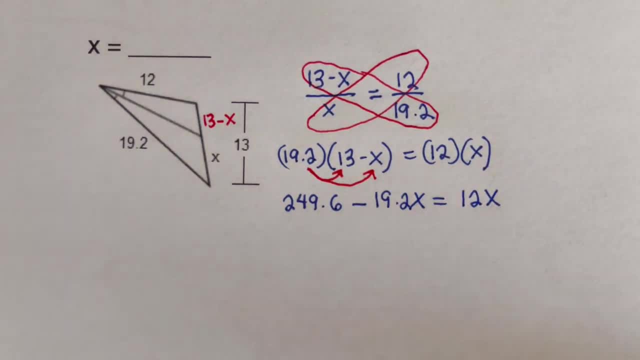 so that we want to solve for x here. so we can go ahead and add um 19.2 from both sides. so plus 19.2 x plus 19.2 x, so that we can cross the 19.2 x out on this side of the equation. so 12 x plus 19.2 x is 31.2 x and we are left with 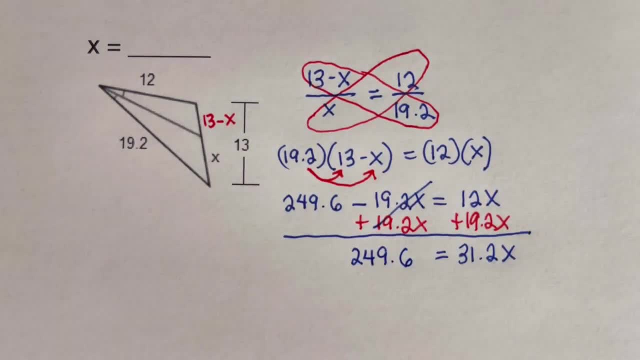 249.6 on this side right here, so that we go ahead and solve for x. so we're going to divide both sides by 31.2. divide this by 31.2 so we can cross this out. we are left with. x is equal to. if we. 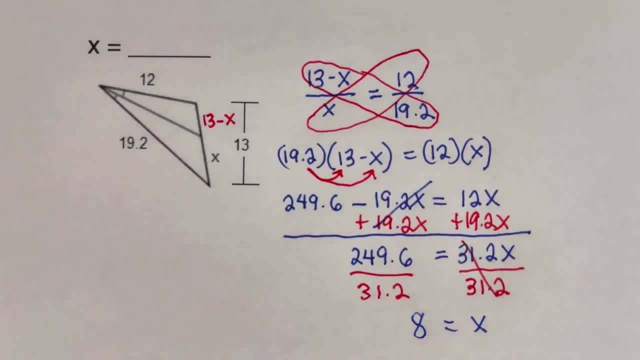 divided them out podcast, we are left with: x is equal to x and if wegame, this is equal to x. well, if we go ahead and divide both sides by 31.2, divide this by 31.2 so we can cross this out, divide these two together, that is equal to eight. so the value of x that we have here is eight. so 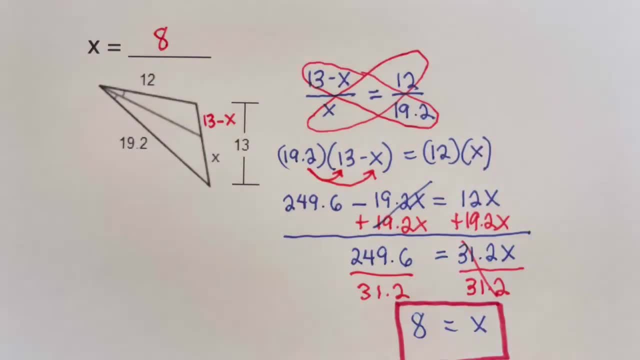 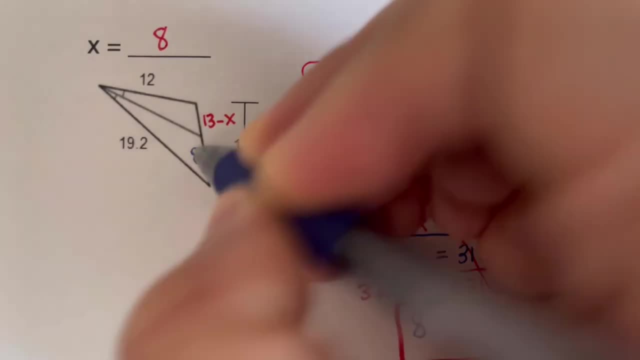 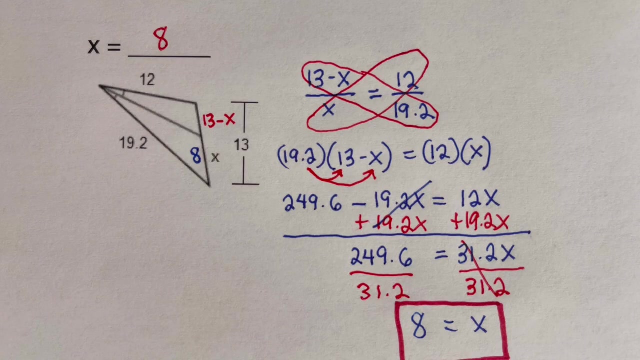 i'm just going to go ahead and put um eight up here. so this means that this corner right here, or this um segment right here is eight and this segment right here from this uh point all the way to that point would be 13 minus x, which is five. so this um segment right here is five. did you get? 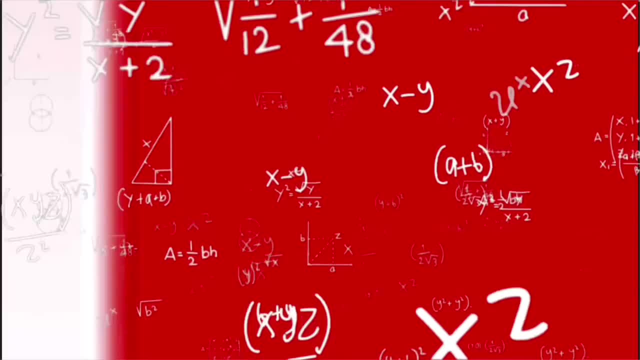 the same answer as this: good, perfect. if you find this video helpful, hit like and subscribe. for more math videos, see ya.